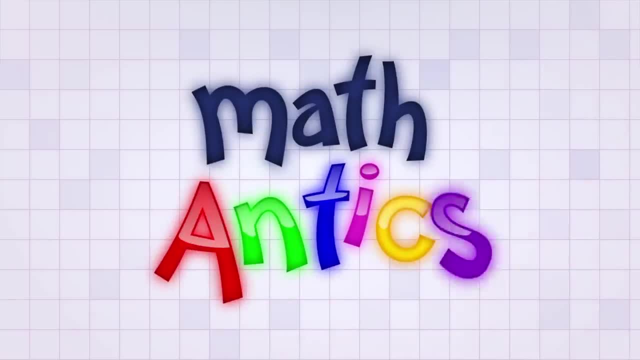 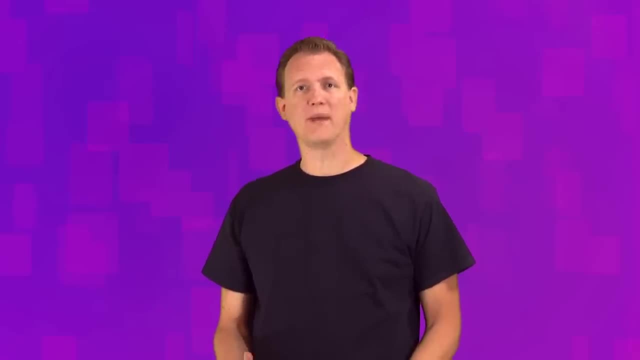 Hi, welcome to Math Antics. In our last video we learned the basics of multi-digit multiplication. We learned how to multiply a multi-digit number by a one-digit number. But in this video we're going to take it to the next level. 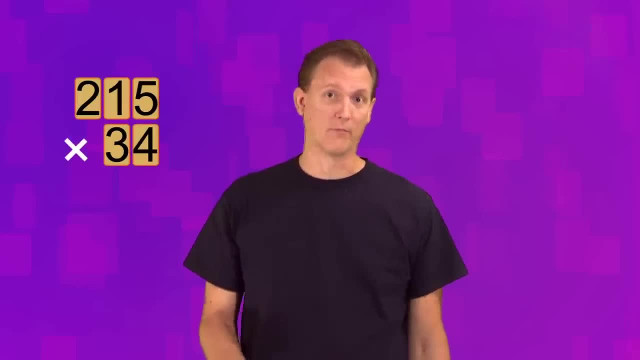 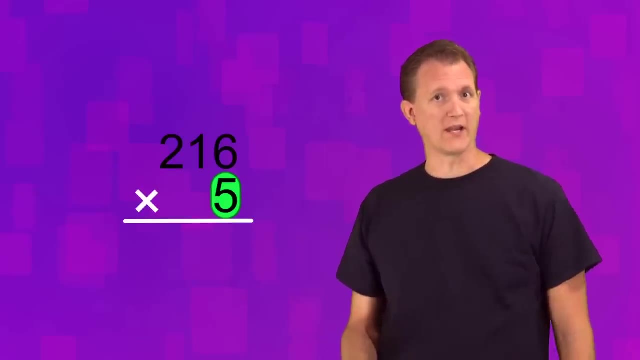 We're going to learn how to multiply a multi-digit number by another multi-digit number. You remember the procedure for multiplying when we have a one-digit bottom number, right? You break up the problem into a series of multiplication steps, one for each of the top digits. 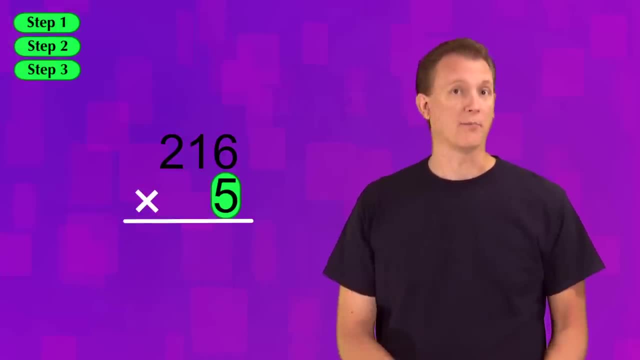 And in each step you just multiply the bottom digit by a top digit, starting with the ones place and working your way left until you've multiplied all of the digits. Well, when the bottom number of your multiplication problem also has more than one digit, 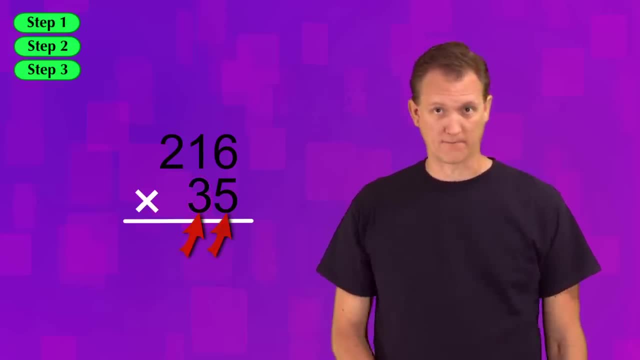 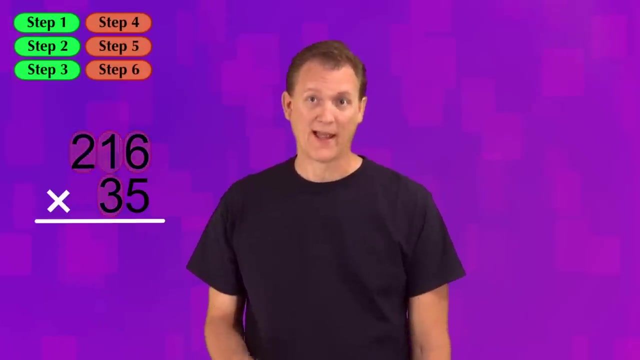 you have to do that same procedure we learned for each bottom digit. For example, if you have a two-digit bottom number, you multiply the first digit by each top digit and then you multiply the second digit by each top digit. That means you're going to have twice as many steps to do and it means you're going to get two different answers. 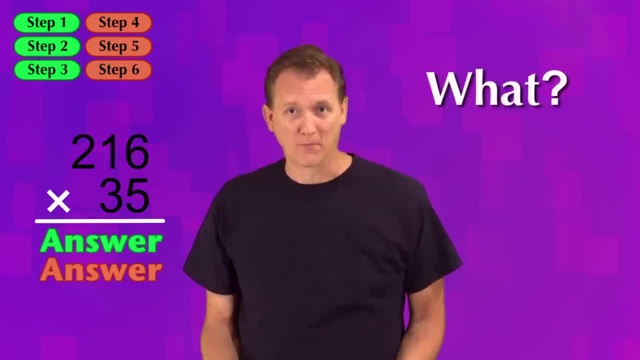 What? How can we have two different answers for the same problem? Now don't panic. The different answers are just what you get from doing the multiplication procedure for each digit of the bottom number separately. In fact, it's kind of like we're pretending we have two separate multiplication problems. 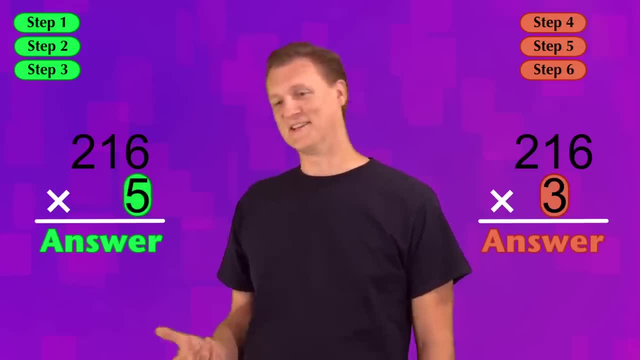 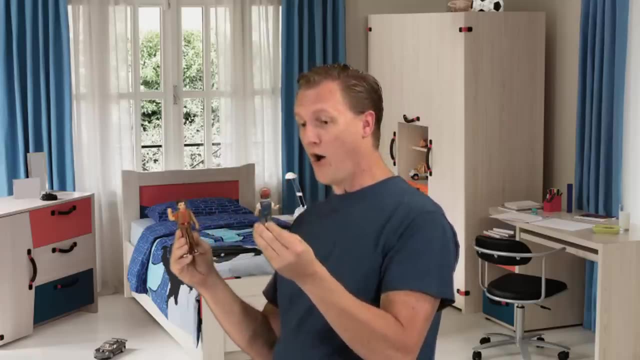 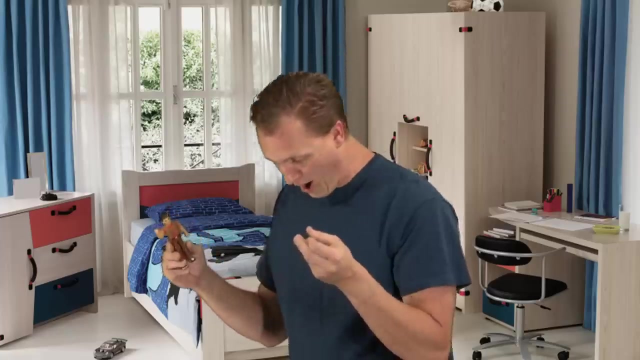 that each have a one-digit bottom number, Which is nice, because I kind of like pretending: No, Luke, I am your father. No, that's impossible. Ha ha, ha. Ah, Wait, no, Noooooo, Ha ha ha. 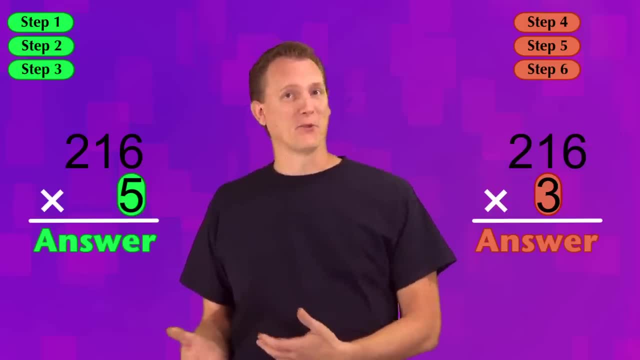 Ugh. well, I mean it's nice because we already know how to do this. Ha ha ha. Well, I mean it's nice because we already know how to do this, because we already know how to multiply when we have a one-digit bottom number. 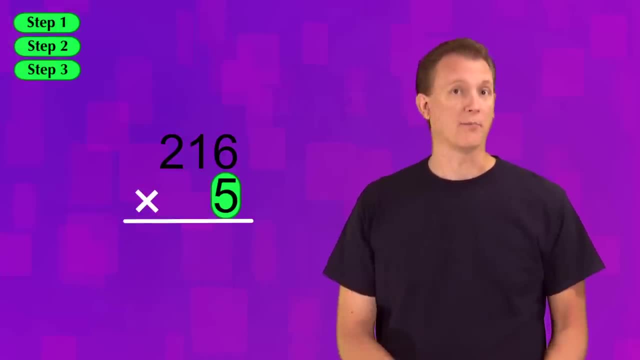 And in each step you just multiply the bottom digit by a top digit, starting with the ones place and working your way left until you've multiplied all of the digits. Well, when the bottom number of your multiplication problem also has more than one digit, 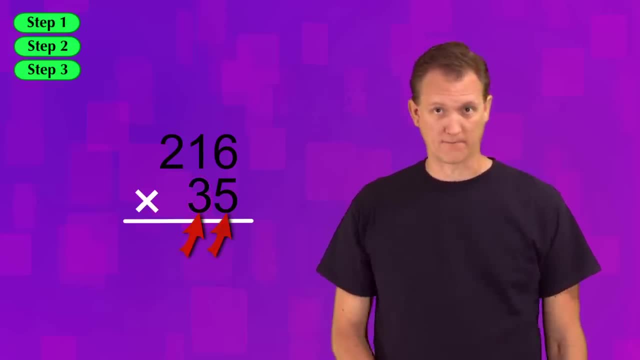 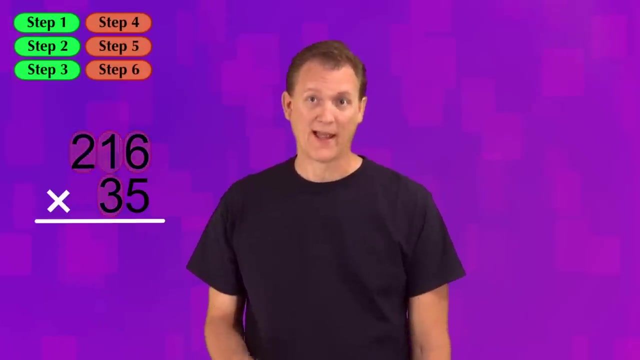 you have to do that same procedure we learned for each bottom digit. For example, if you have a two-digit bottom number, you multiply the first digit by each top digit and then you multiply the second digit by each top digit. That means you're going to have twice as many steps to do and it means you're going to get two different answers. 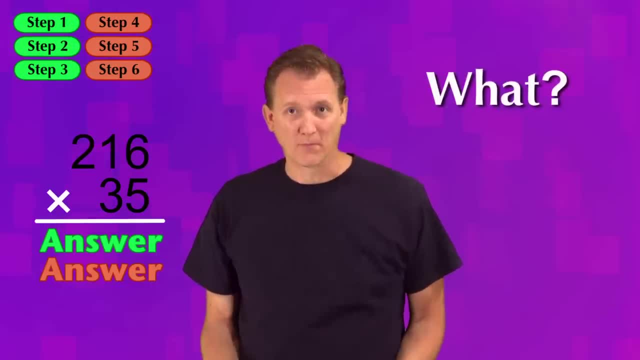 What? How can we have two different answers for the same problem? Now don't panic. The different answers are just what you get from doing the multiplication procedure for each digit of the bottom number separately. In fact, it's kind of like we're pretending we have to separate multiplication problems. 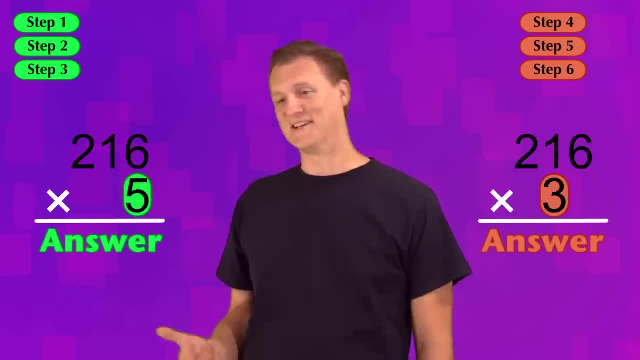 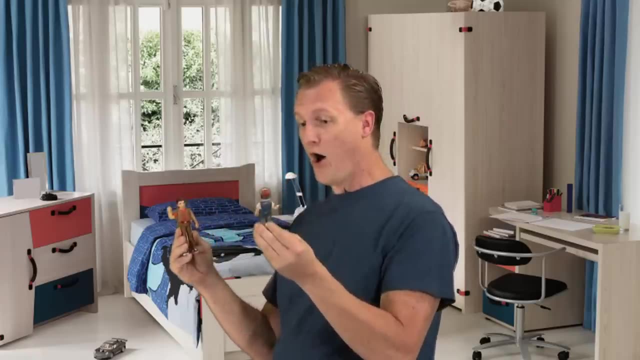 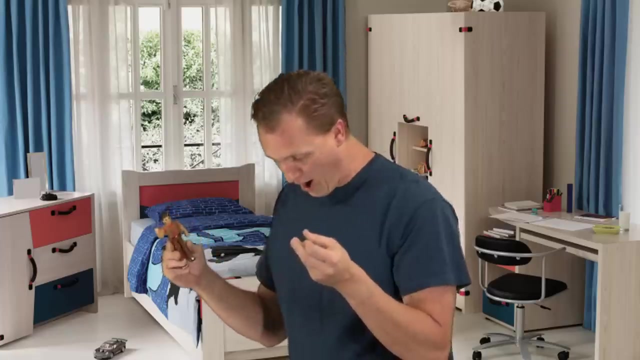 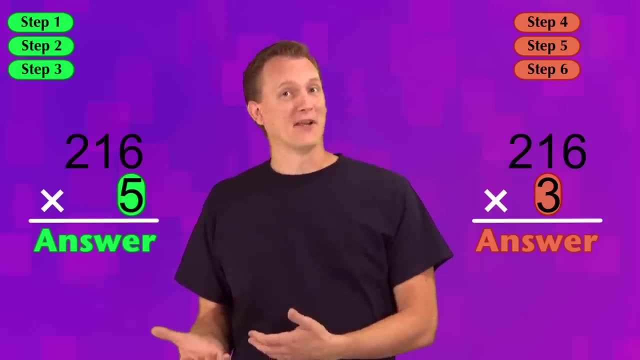 that each have a one-digit bottom number, Which is nice, cuz I kind of like pretending: No, Luke, I am your father. No, That's impossible, Ha. Haha. Well, I mean it's nice because we already know that theığım. 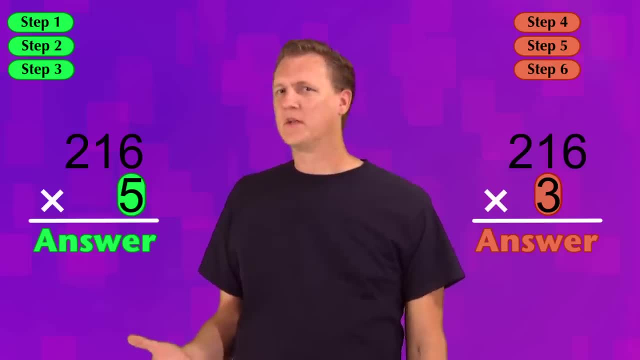 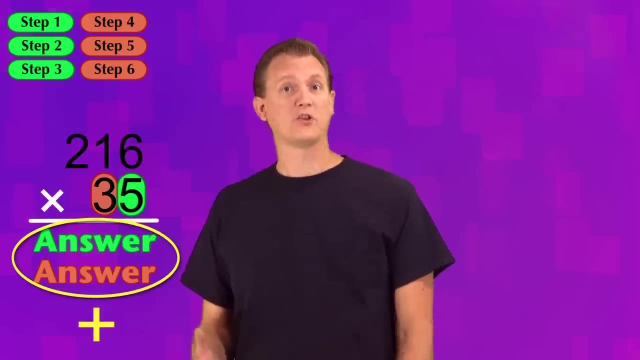 how to multiply when we have a one-digit bottom number. But then what will we do with the two different answers we're going to get? Well, it turns out that all we have to do is add them together once we're finished doing all of our multiplication steps. 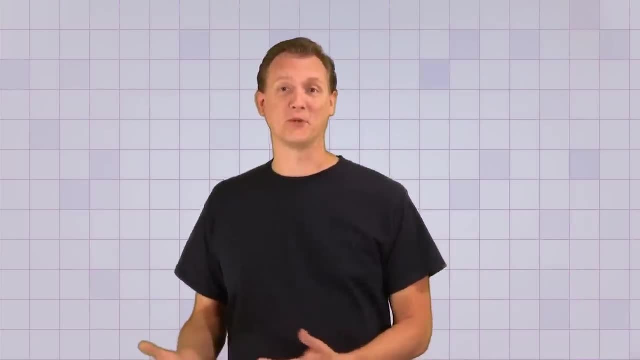 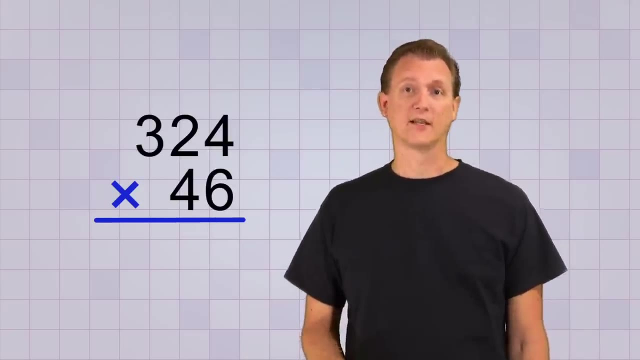 Are you ready to see an example? It should make a lot more sense when you see the procedure in action. So let's multiply 324 by 46. Now remember we're going to do the same procedure that we did in the last video. 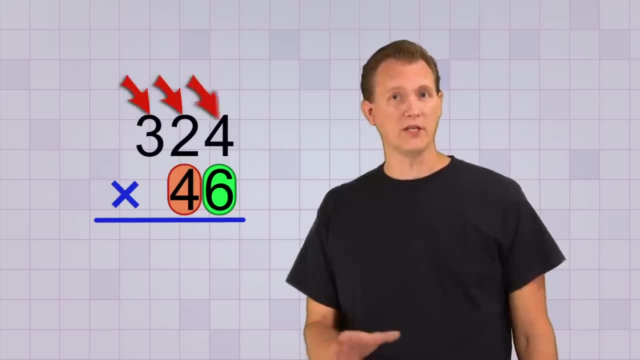 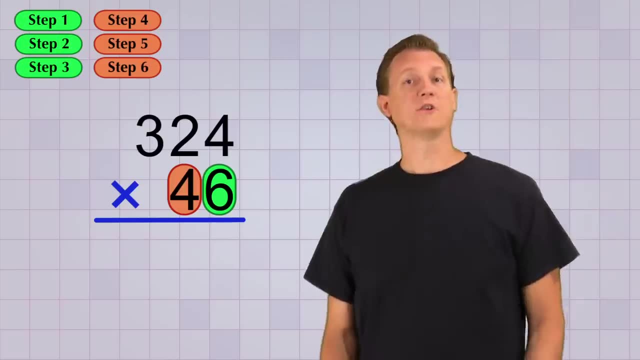 for each of the bottom digits And since our top number has three digits, that means there'll be three multiplication steps for the first digit and three steps for the second digit. Fortunately, we can start the same way we would if the bottom number only had one digit. 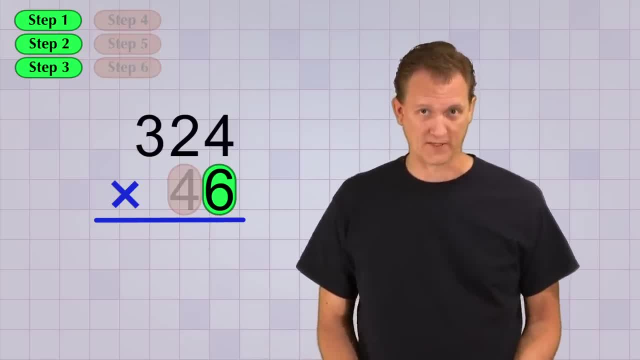 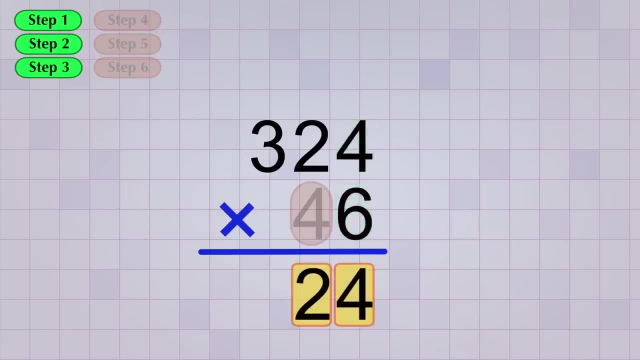 by just ignoring the second digit until we finish the first three steps. Alright, so our first multiplication step is 6 times 4, which is 24.. And since 24 has two digits, we can leave the 4 in our answer line. 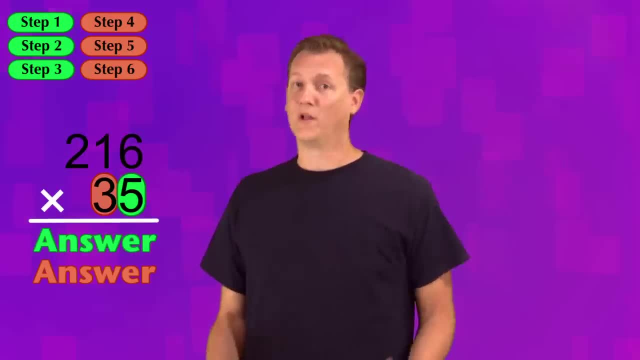 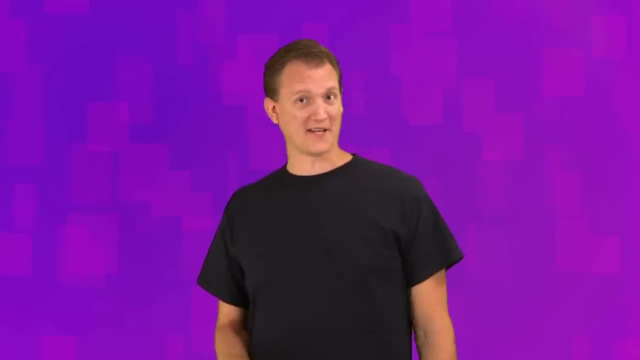 But then what will we do with the two different answers we're going to get? Well, it turns out that all we have to do is add them together once we're finished doing all of our multiplication steps. Are you ready to see an example? 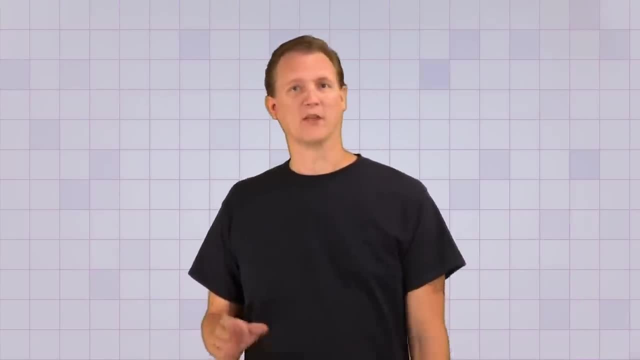 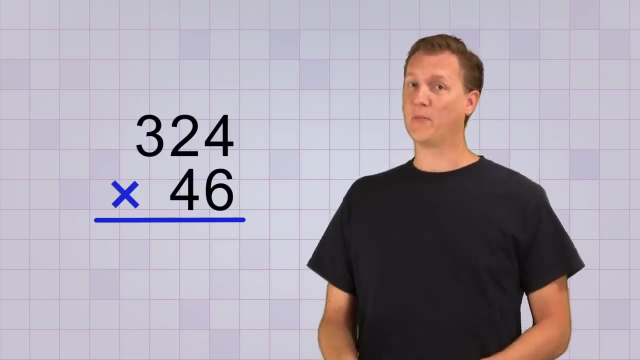 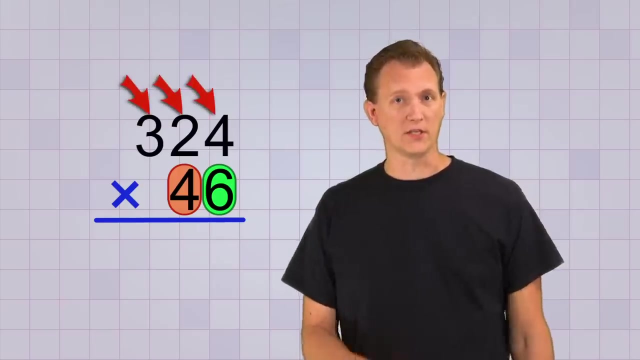 It should make a lot more sense when you see the procedure in action. So let's multiply 324 by 46. Now, remember, we're going to do the same procedure that we did in the last video for each of the bottom digits And since our top number has 3 digits, 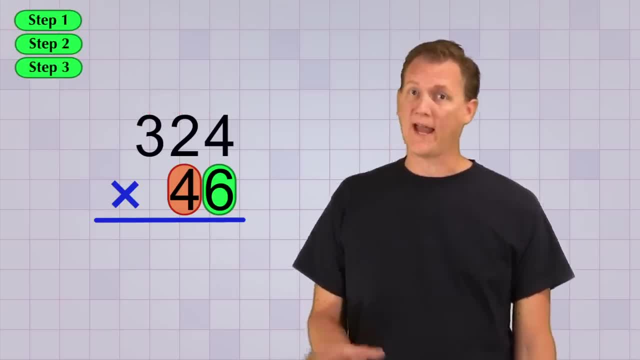 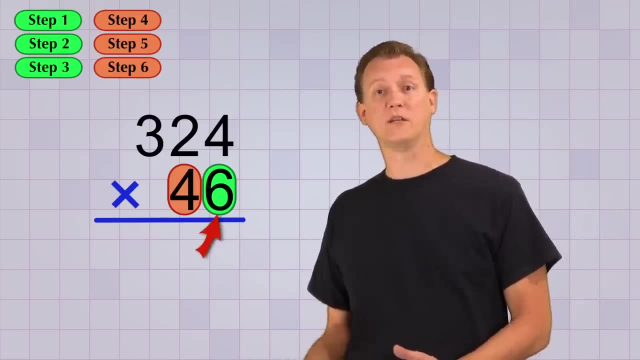 that means there'll be 3 multiplication steps for the first digit and 3 steps for the second digit. Fortunately, we can start the same way we would if the bottom number only had 1 digit, by just ignoring the second digit until we finish the first 3 steps. 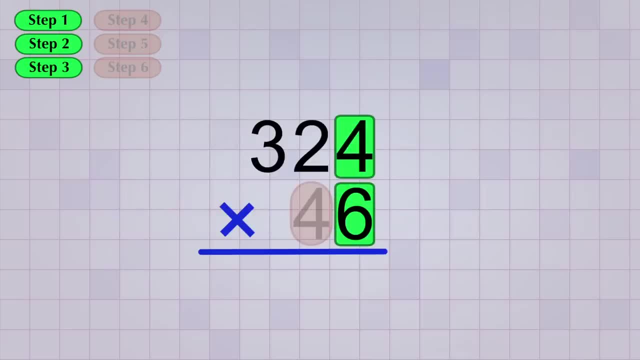 Alright, so our first multiplication step is 6 times 4, which is 24.. And since 24 has 2 digits, we can leave the 4 in our answer line, but we need to carry the 2 and put it above the next top digit that we're going to multiply. 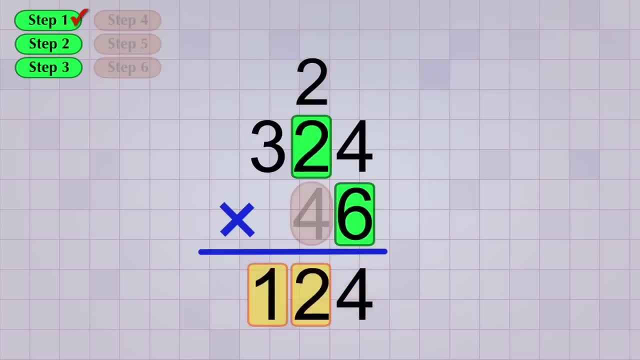 So the next step is 6 times 2, which is 12.. But we have to add in the 2 that we carried. so 12 plus 2 gives us 14.. That's another 2-digit answer. so we leave the 4 in our answer line. 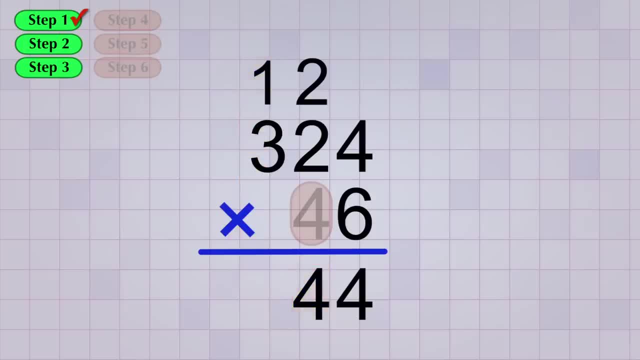 and carry the 1 up above the next digit that we're going to multiply, And our third step is 6 times 3, which is 18, and then we add in the 1 that we carried and we get 19.. This time we can leave both digits of the 19 in our answer line. 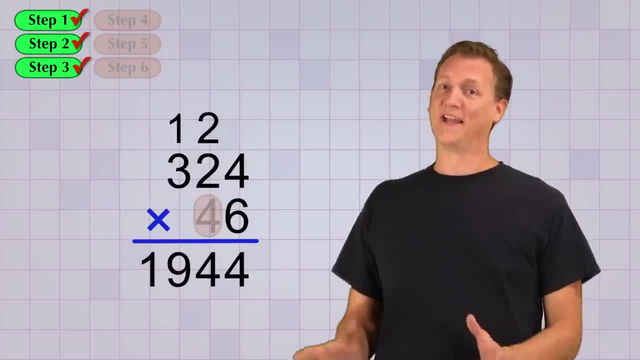 because there's no more multiplication steps to do. Well, at least there's no more steps for the first digit. Remember, we still have that other bottom digit that we've been ignoring. Now we have to multiply it by each of the top digits also. 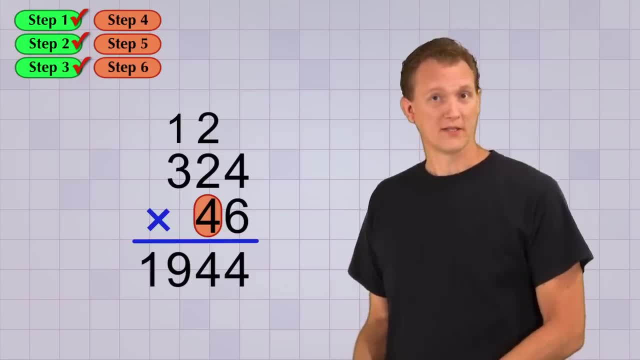 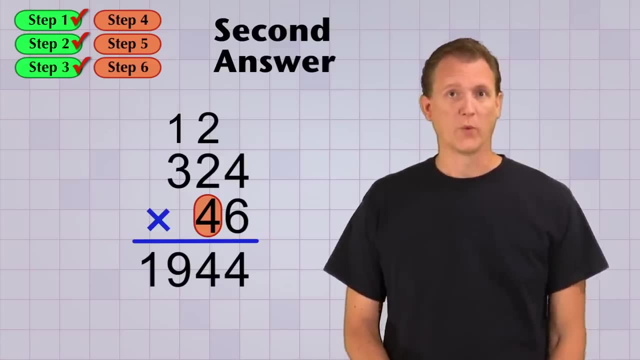 which means we have 3 more steps to do. It also means that we'll get a second answer, And because we'll get a second answer, we need to start a second answer line for the next set of steps. We're going to put our new answer line just below the first one. 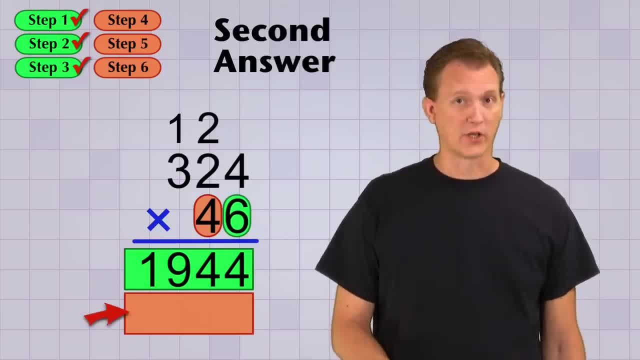 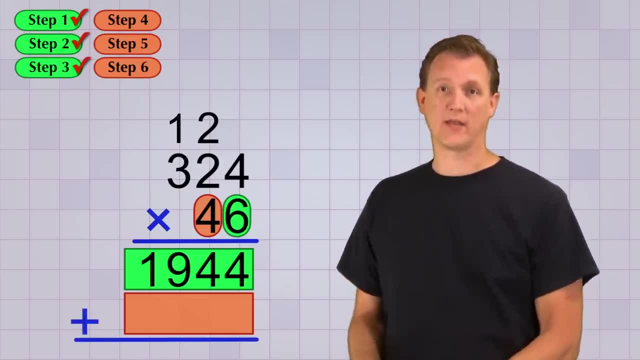 So this answer line comes from our first bottom digit and this answer line will come from our second bottom digit At the very end. after we're all done multiplying, we're going to add the two answers together, But for now let's continue with the second set of multiplication steps. 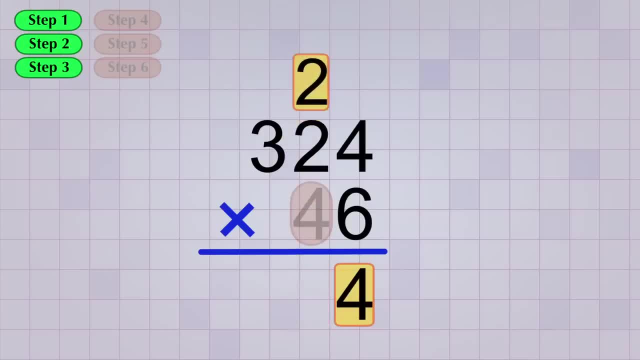 but we need to carry the 2 and put it above the next top digit that we're going to multiply. So the next step is 6 times 2, which is 12.. But we have to add in the 2 that we carried. so 12 plus 2 gives us 14.. 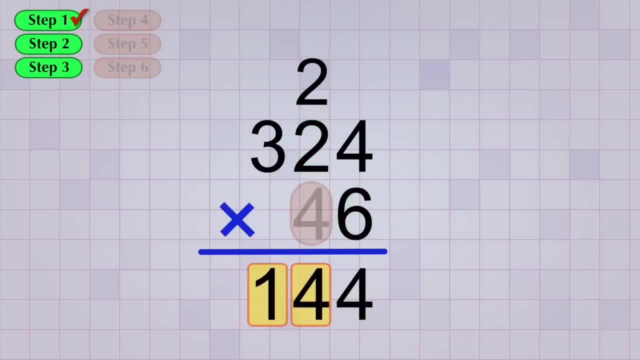 That's another two-digit answer. so we leave the 4 in our answer line and carry the 1 up above the next digit that we're going to multiply And our third step is 6 times 3, which is 18, and then we add in the 1 that we carried and we get 19.. 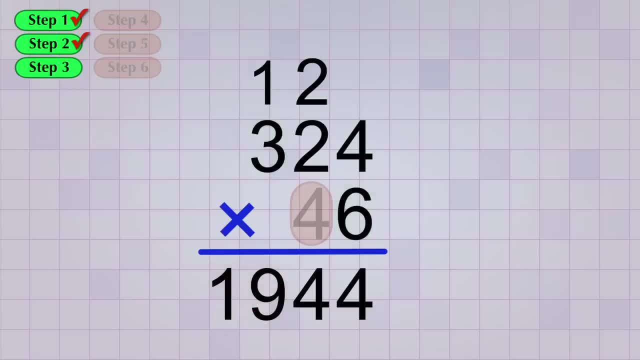 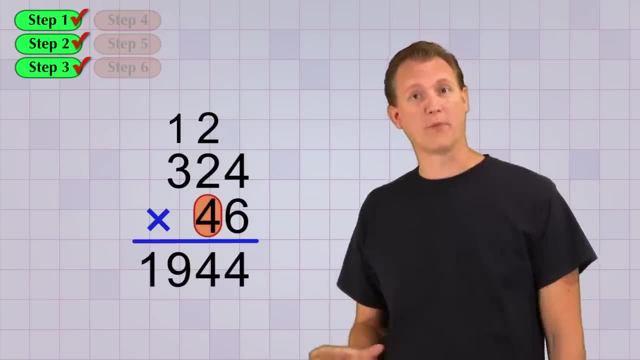 This time we can leave both digits of the 19 in our answer line because there's no more multiplication steps to do. Well, at least there's no more steps for the first digit. Remember, we still have that other bottom digit that we've been ignoring. 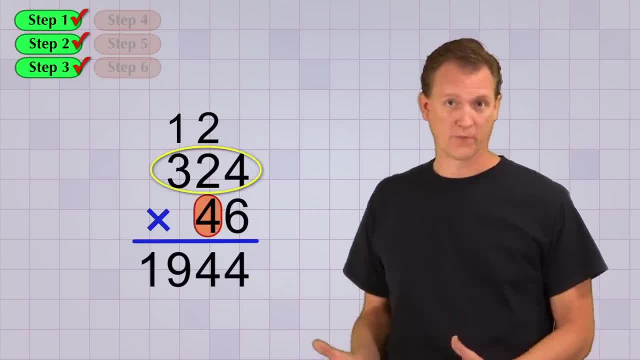 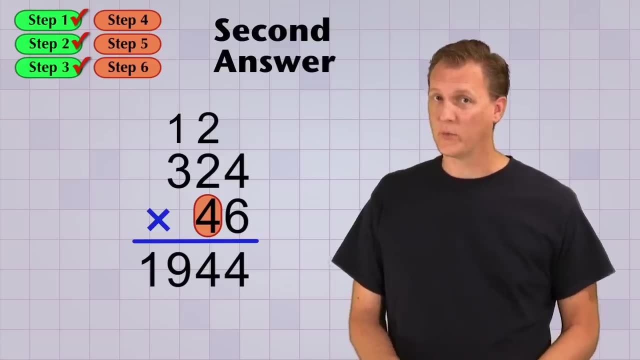 Now we have to multiply it by each of the top digits also, which means we have three more steps to do. It also means that we'll get a second answer, And because we'll get a second answer, we need to start a second answer line for the next set of steps. 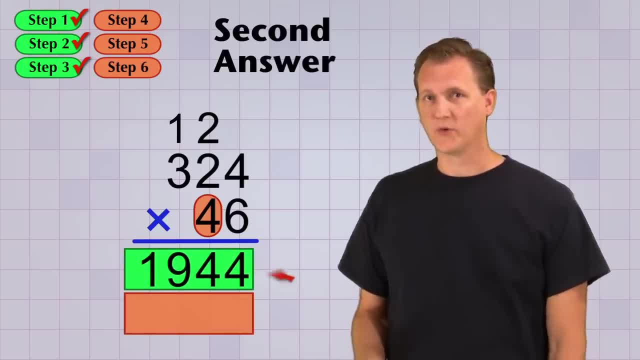 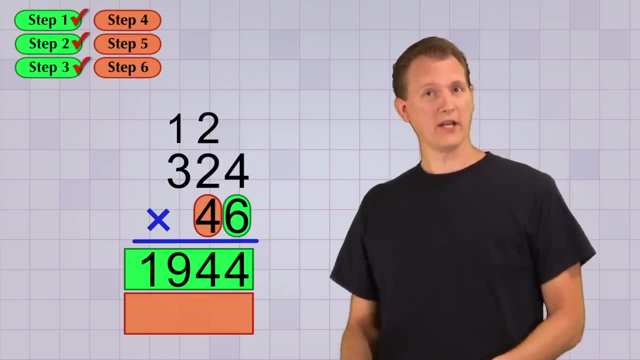 We're going to put our new answer line just below the first one, So this answer line comes from our first bottom digit and this answer line will come from our second bottom digit At the very end. after we're all done multiplying, we're going to add the two answers together. 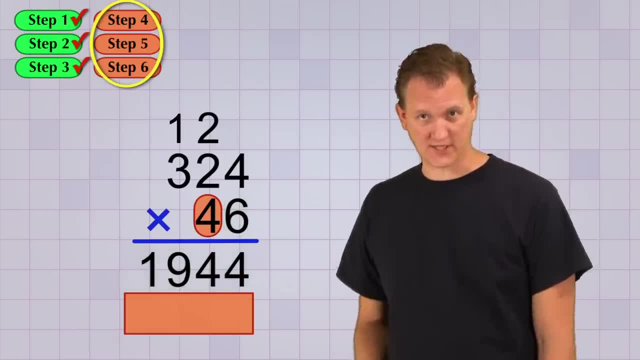 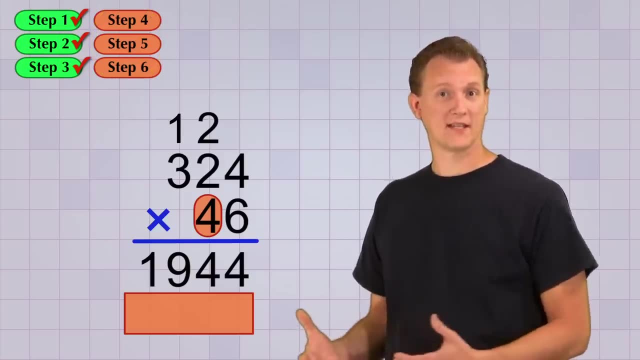 But for now, let's continue with the second set of multiplication steps. Oh, and I almost forgot to tell you, there's something very important that you need to do when you start the second set of steps, Because the second digit of the bottom number is in the tens place. 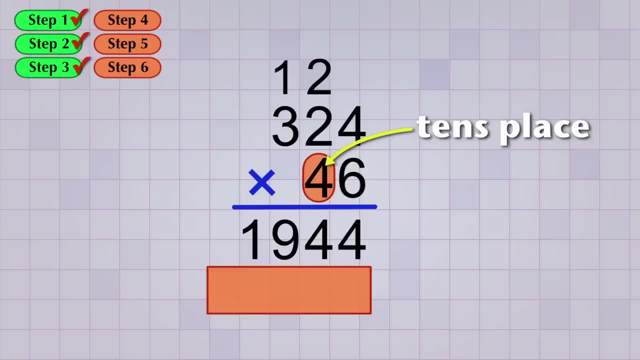 that means that even though the digit's only a 4, its value is really 40. That's 10 times bigger, so the answer we get should also be 10 times bigger. So before we start multiplying we need to put a zero in the first spot of our answer line. 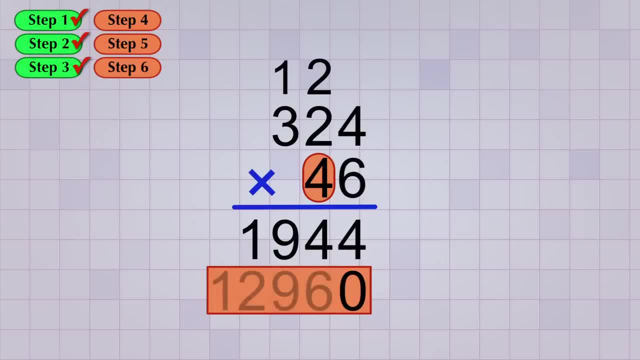 so it's 10 times bigger. That means that all the other answer digits we put there are shifted to the next bigger number place And just so you know, if we happen to have a third bottom digit, we would get a third answer line. 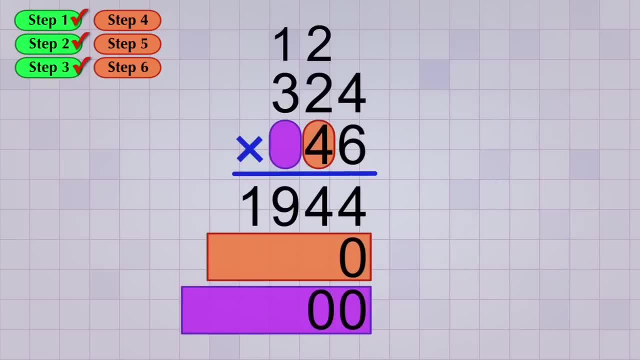 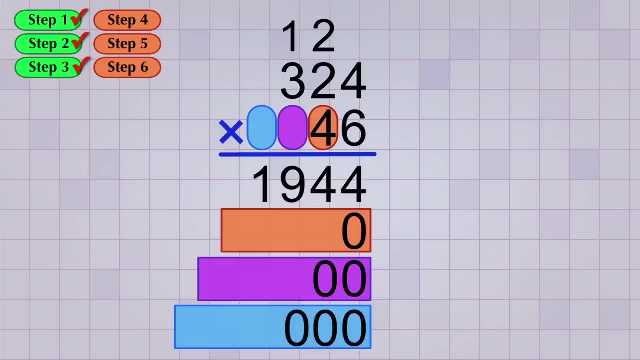 and we need to shift the third answer over by two zeros because it would be 100 times bigger. And if we add a fourth digit, there'd be a fourth answer line shifted over by three zeros. And if we add a fifth bottom digit, 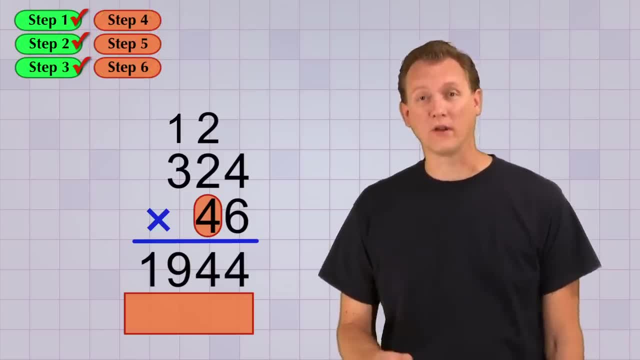 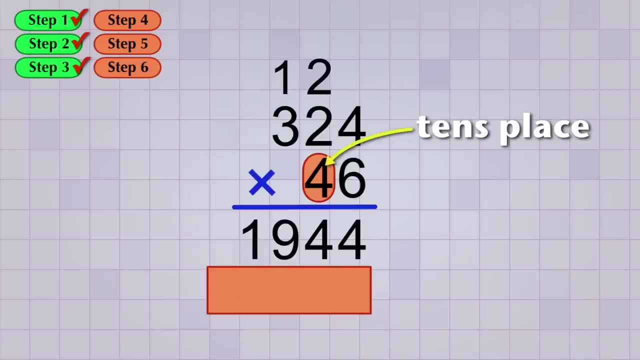 Oh, and I almost forgot to tell you. there's something very important that you need to do when you start the second set of steps, Because the second digit of the bottom number is in the tens place. that means that even though the digit's only a 4, its value is really 40.. 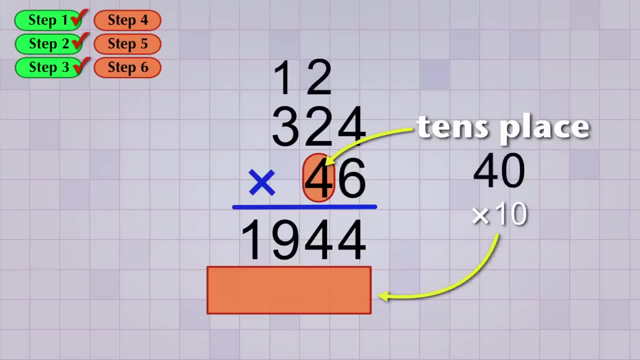 That's 10 times bigger and the answer we get should also be 10 times bigger. So before we start multiplying we need to put a zero in the first spot of our answer line. so it's 10 times bigger. That means that all the other answer digits we put there. 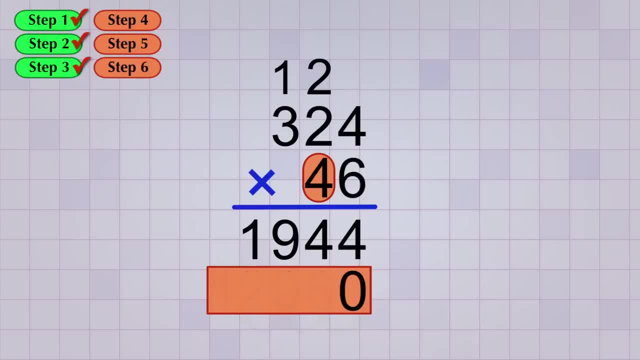 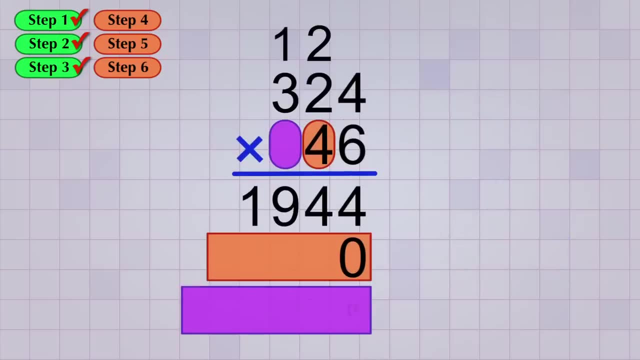 are shifted to the next bigger number place. And just so you know, if we happen to have a third bottom digit, we would get a third answer line and we need to shift the third answer over by two zeros because it would be 100 times bigger. 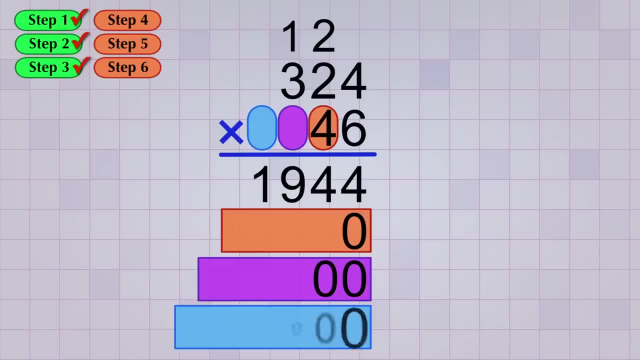 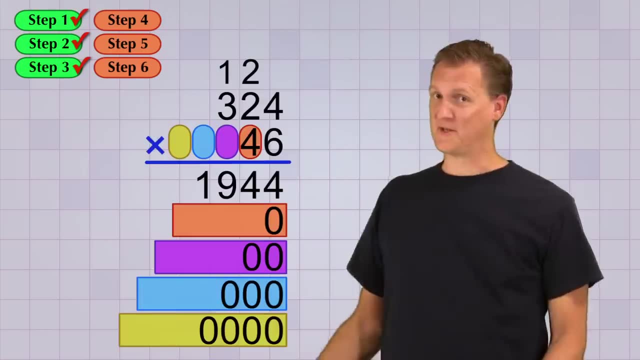 And if we add a fourth digit, there'd be a fourth answer line shifted over by three zeros. And if we add a fifth bottom digit, there'd be a fifth answer line shifted over by four zeros. See the pattern. Boy am I glad we've only got two bottom digits. 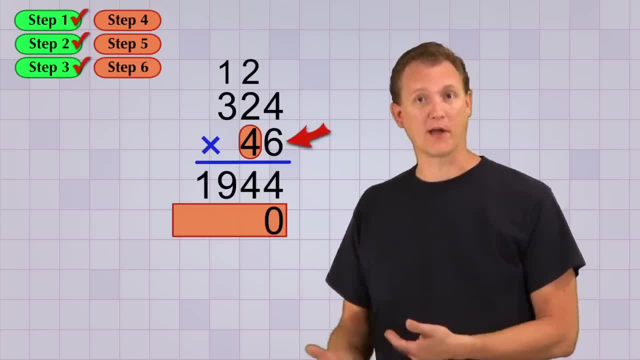 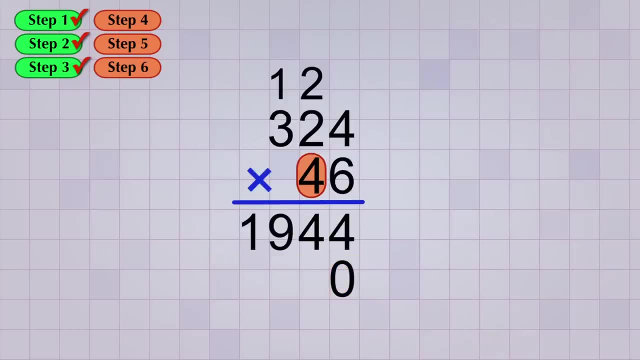 And now you see why we always put the number with the fewest digits on the bottom when we're multiplying. But let's continue with our problem. Let's do the first step of our second bottom digit. We multiply that digit 4,. 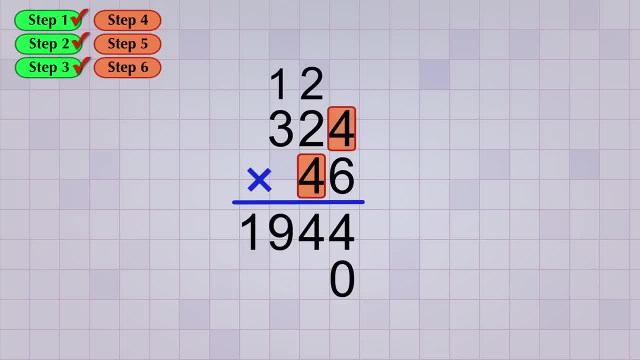 by the ones place digit of the top number, which is also a 4.. 4 times 4 equals 16, and that goes in our second answer line, right next to the extra zero we put there. Now, remember, because 16 is a two digit answer. 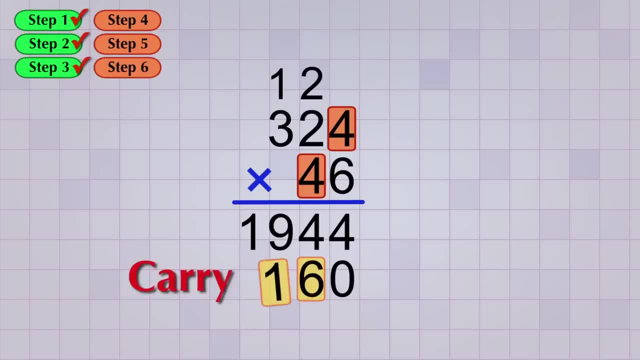 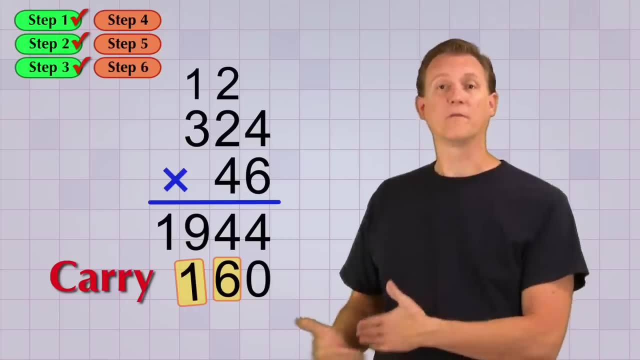 we have to carry And we always put the digit we carry above the next top digit. that we'll multiply. But before we can carry it up to that place we need to cross out all the digits that we carried from our first answer line. 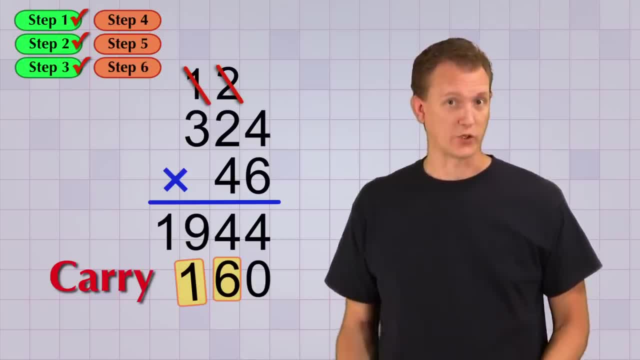 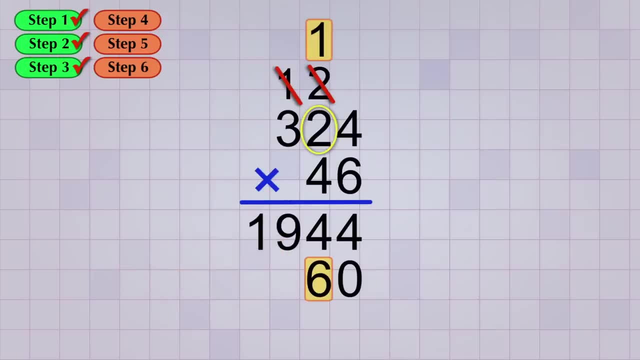 because we've already used them. We don't want to accidentally add them to our second answer line There. So now we can carry our 1 to the top of the tens place, which means it will go in the column above this 2,. 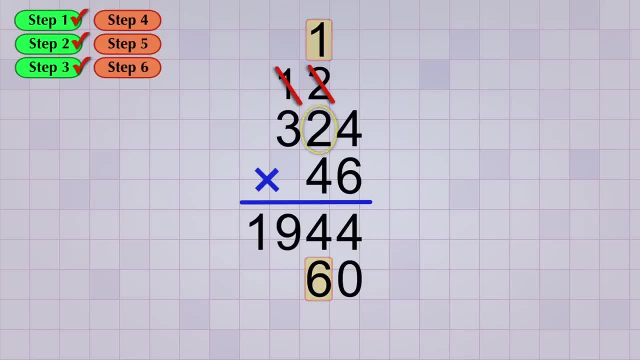 because that's the next top digit that we'll multiply with our bottom digit. Now we can do the next multiplication step: 4 times 2 gives us 8, and then we'll add the 1 that we carried and we get 9.. 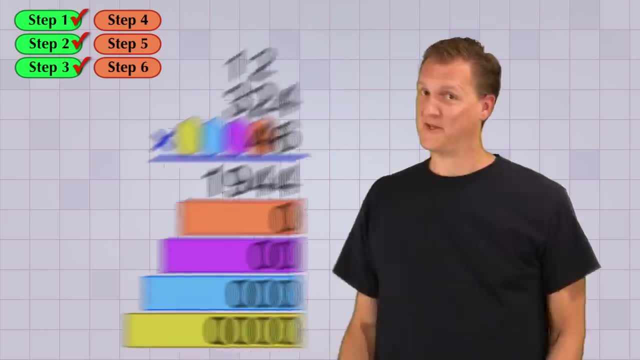 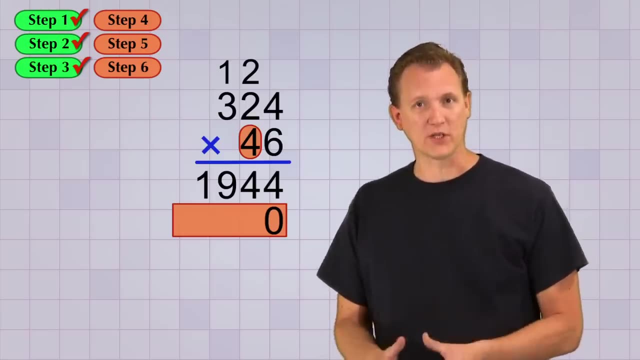 there'd be a fifth answer line shifted over by four zeros. See the pattern. Boy, am I glad we've only got two bottom digits. And now you see why we always put the number with the fewest digits on the bottom when we're multiplying. 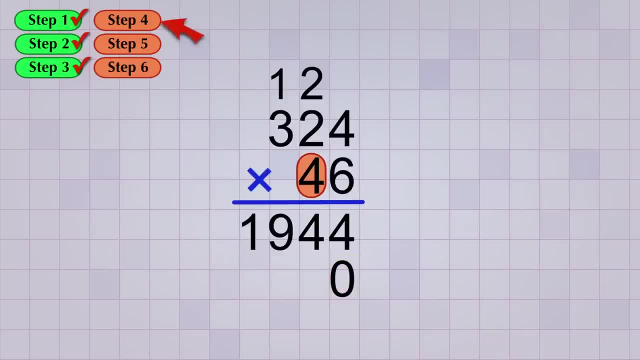 But let's continue with our problem. Let's do the first step of our second bottom digit. We multiply that digit- 4, by the ones place digit of the top number, which is also a 4.. 4 times 4,. 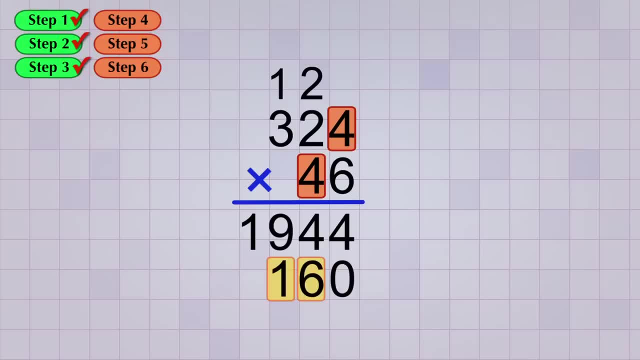 gives us 16, and that goes in our second answer line, right next to the extra zero we put there. Now, remember, because 16 is a two digit answer we have to carry And we always put the digit we carry above the next top digit. that we'll multiply. 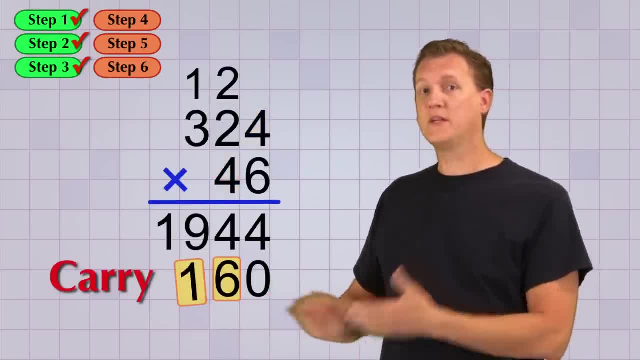 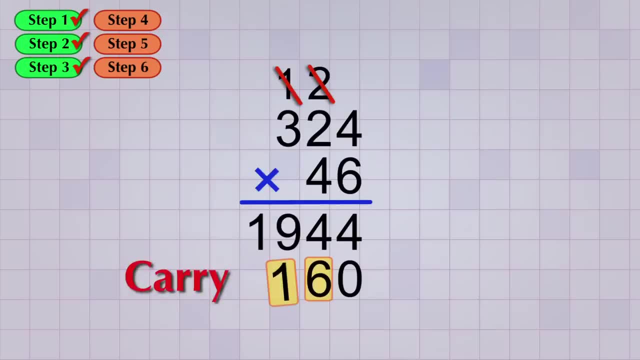 But before we can carry it up to that place we need to cross out all the digits that we carried from our first answer line because we've already used them. We don't want to accidentally add them to our second answer line There. 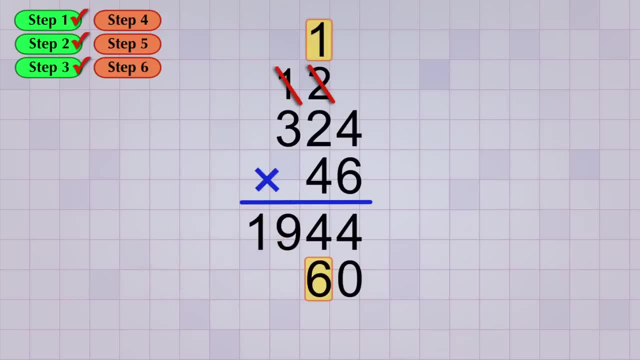 So now we can carry our 1 to the top of the tens place, which means it will go in the column above this 2, because that's the next top digit that we'll multiply with our bottom digit. Now we can do the next multiplication step. 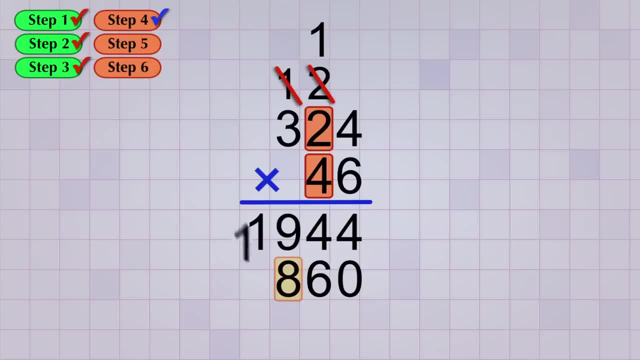 4 times 2 gives us 8, and then we'll add the 1 that we carried and we get 9.. Great, Finally a one digit answer. so we don't have to carry this time. We just write the 9 in the next place of our answer line. 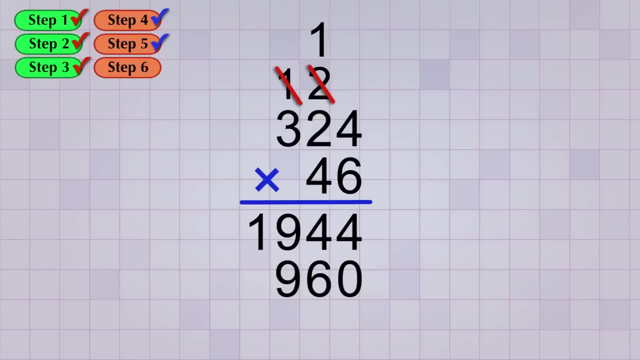 and move on to the next step. The next and last multiplication step is 4 times 3,, which is 12.. And since there's no more steps, we can write both digits in our second answer line. Alright, We're finally done with all our multiplication steps. 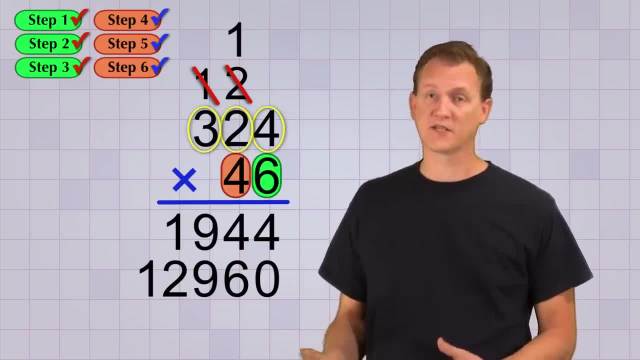 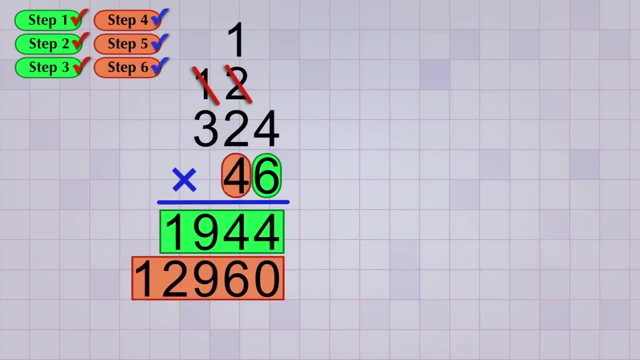 We multiplied each bottom digit by each top digit, just like we were supposed to. But now what do we do? We have two answer lines, but this is just one multiplication problem. Well, remember, the reason we have two answer lines is that we're pretending that we're doing. 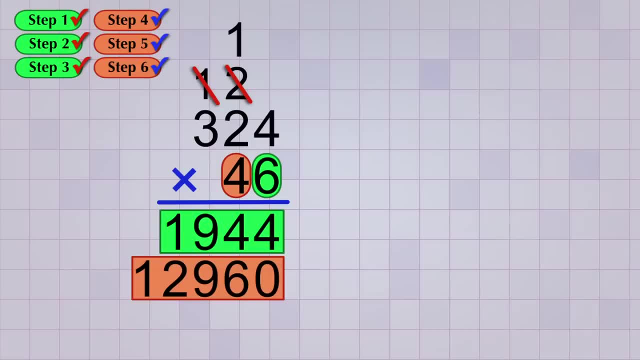 two separate multiplication problems. We treated it like it was 6 times 324, and 4 times 324.. But since the 4 was in the tens place, we had to put an extra zero in our second answer, since it would really be the answer from 40 times 324.. 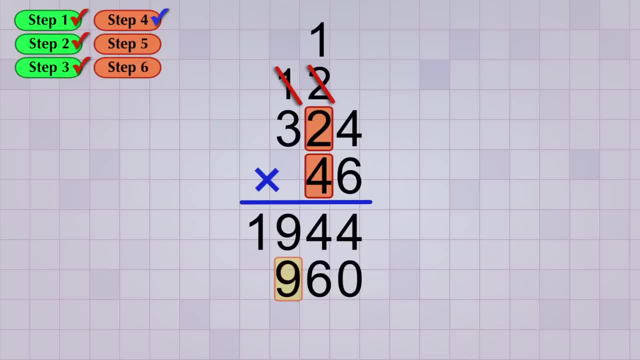 Great, Finally a one digit answer. so we don't have to carry this time. We just write the 9 in the next place of our answer line and move on to the next step. The next multiplication step is 4 times 3,. 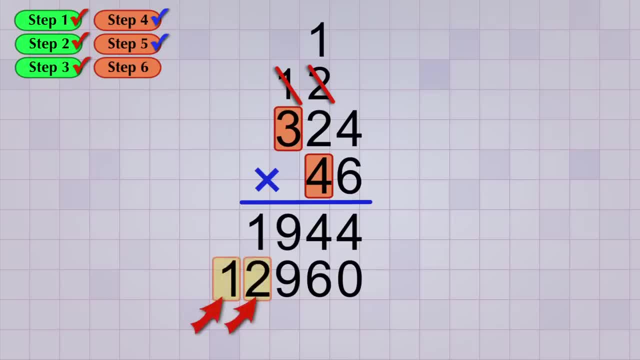 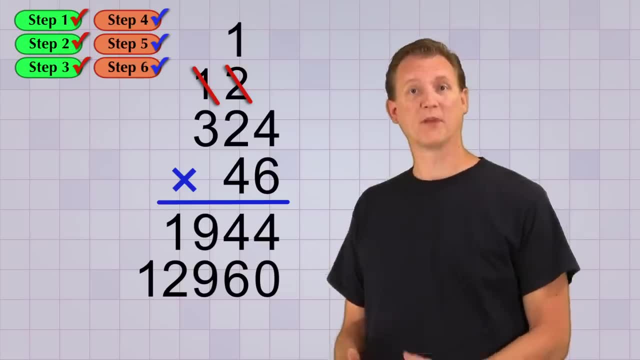 which is 12.. And since there's no more steps, we can write both digits in our second answer line. Alright, we're finally done with all our multiplication steps. We multiplied each bottom digit by each top digit, just like we were supposed to. 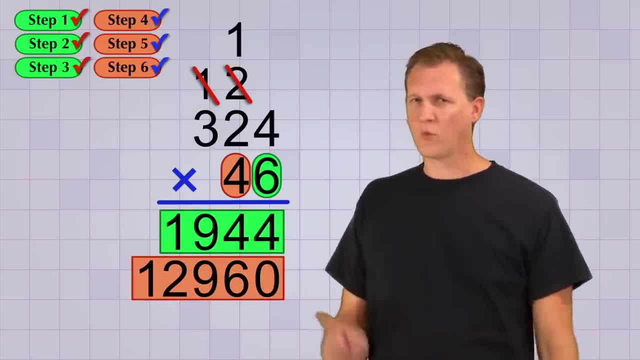 But now what do we do? We have two answer lines, but this is just one multiplication problem. Well, remember, the reason we have two answer lines is that we're pretending that we're doing two separate multiplication problems. We treated it like it was 6 times 324 and 4 times 324.. 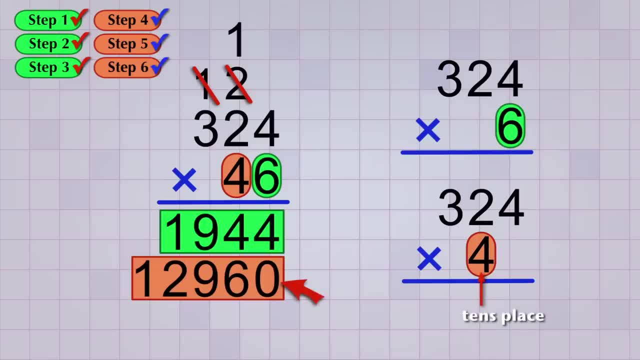 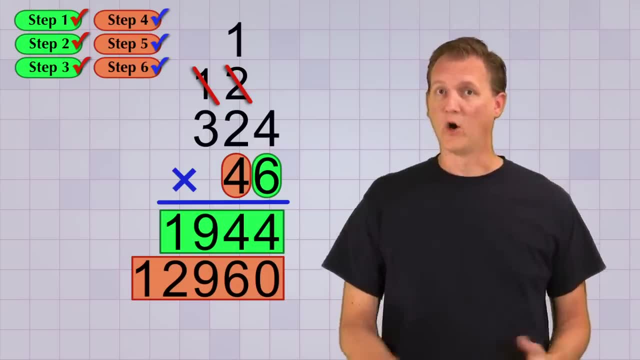 But since the 4 was in the tens place, we had to put an extra zero in our second answer, since it would really be the answer from 40 times 324.. Now, as I mentioned earlier, all we have to do to get the final answer. 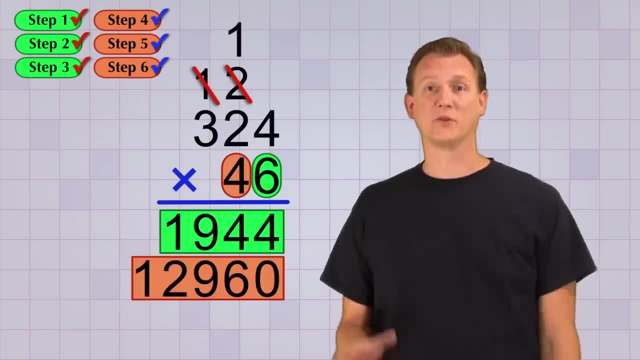 is, add those two answers together, And the great news is that those answers are already stacked up, like an addition problem should be, so we can just draw a line below them and stick a plus sign on the left side. Now we can add them column by column. 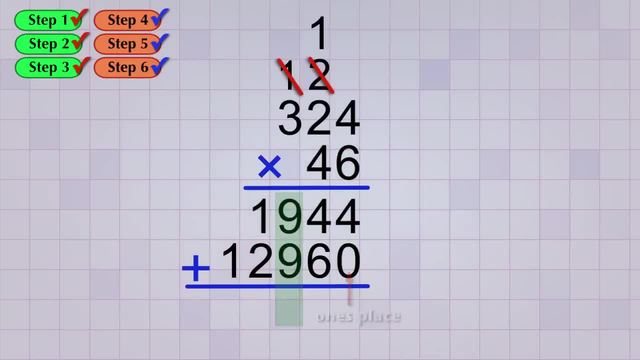 starting from the ones place, just like we did in the multi-digit addition video. 4 plus 0 equals 4.. 4 plus 6 equals 10, so we carry the 1.. 1 plus 9 plus 9 equals 19,, so we carry the 1 again. 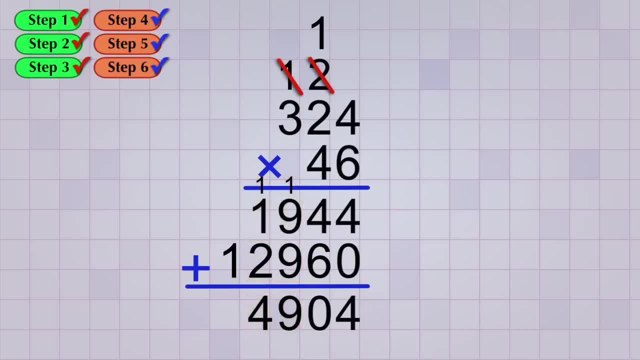 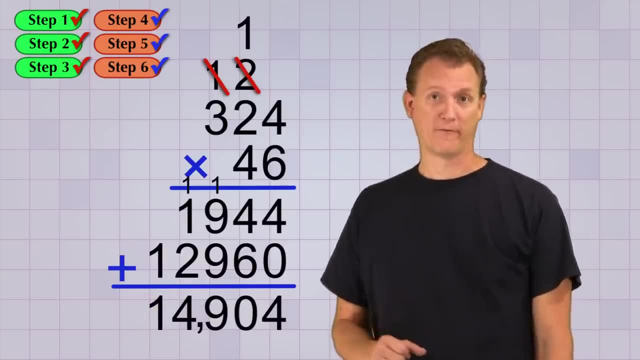 1 plus 1 plus 2 equals 4.. And then our last answer, digit is just 1.. There, our final answer is a pretty big number: 14,904.. Let's double-check with a calculator to make sure we got it right. 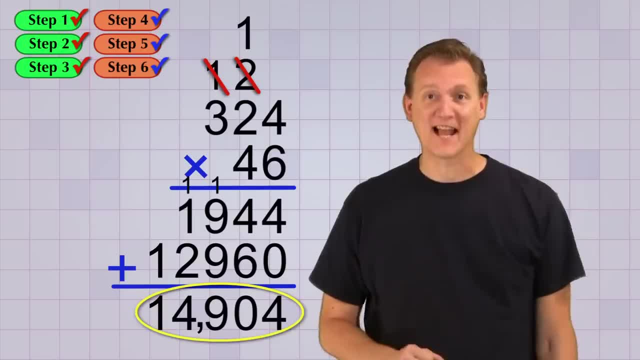 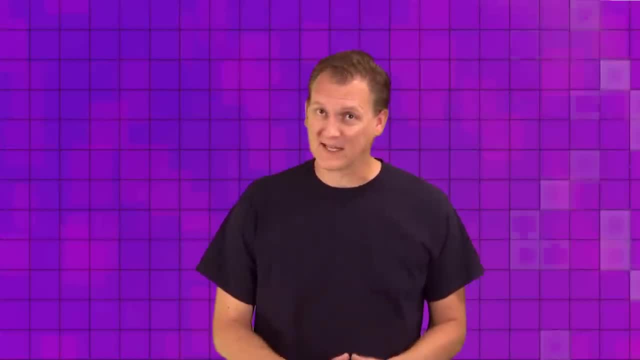 Let's see. Yep, That's exactly what you get when you multiply 324 by 46.. OK, I know that procedure is kinda complicated, so don't get frustrated if you don't get it right away. Just take some time and practice to really get the hang of it. 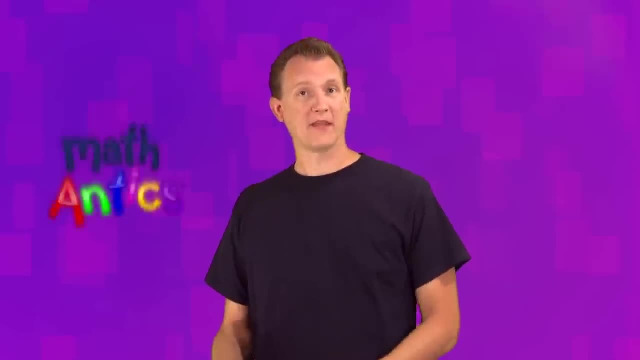 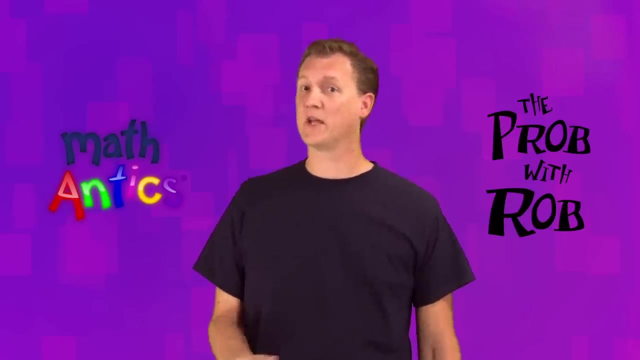 And you can always re-watch this video if you need to, And if you're a Math Antics subscriber, be sure to check out the extra problems I work through in the Prob with Rob video examples. After that, you can try some of the exercises on your own. 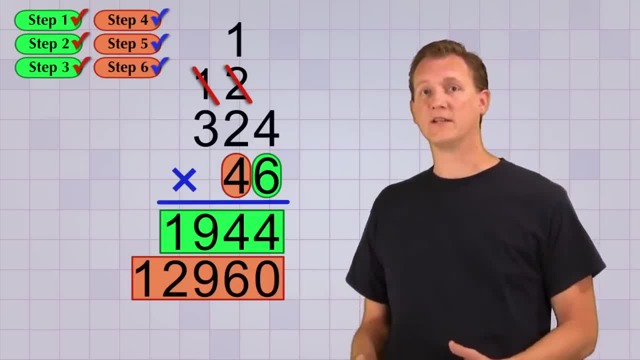 Now, as I mentioned earlier, all we have to do to get the final answer is add those two answers together, And the great news is that those answers are already stacked up, like an addition problem should be, so we can just draw a line below them.